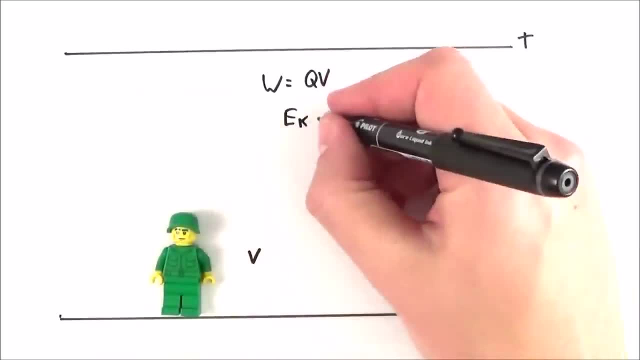 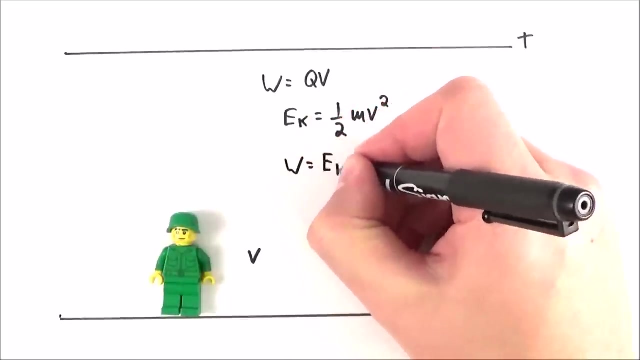 time it hits the bottom And we can say that kinetic energy is going to be equal to a half m v squared. Now, the amount of work we do on it is the amount of electrical potential it has at the start, And if that's 100% efficient, we can say that the work done all ends up as kinetic energy. 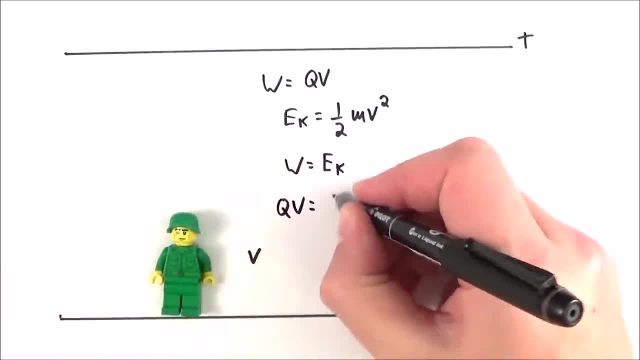 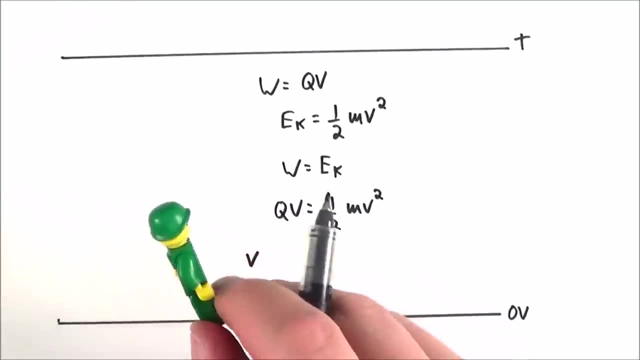 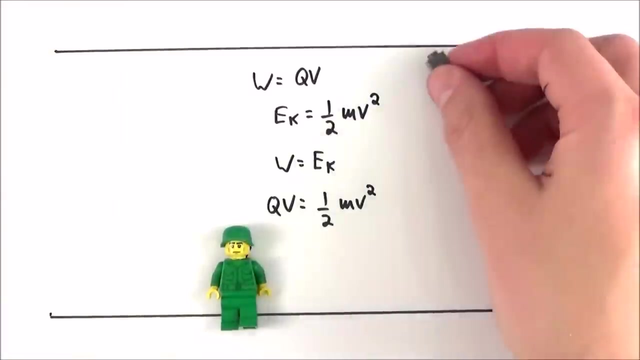 at the end, And therefore qv is going to be equal to a half m v squared. What does that mean? Well, if maybe, rather than having something which is maybe just a unit charge, if we had, maybe, an electron. So here we have an electron which has the opposite charge. This wants to be a. 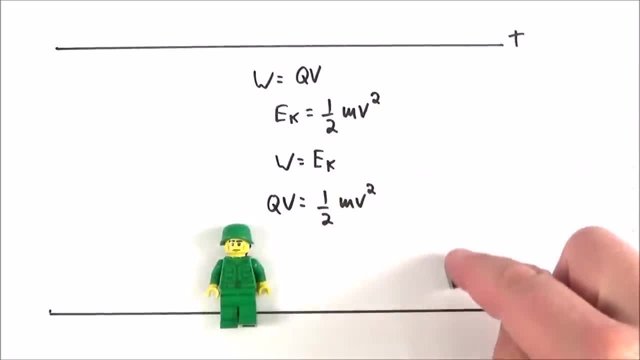 positive end. So we can do work on the electron. We move it away And as soon as we let it go, if it's free to move, it's going to accelerate towards the positive plate. Now the charge on the electron: we give the symbol e. This is the elementary charge of minus 1.6 times 10 to minus. 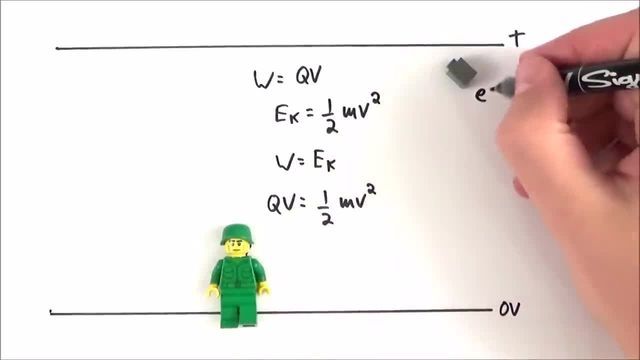 19 coulombs, And the energy it's going to need to do to get it out there is going to be equal to e times the potential difference that we've moved it through, And this can then turn into its kinetic energy, which equals a half m v squared, And you might notice some similarities between this and 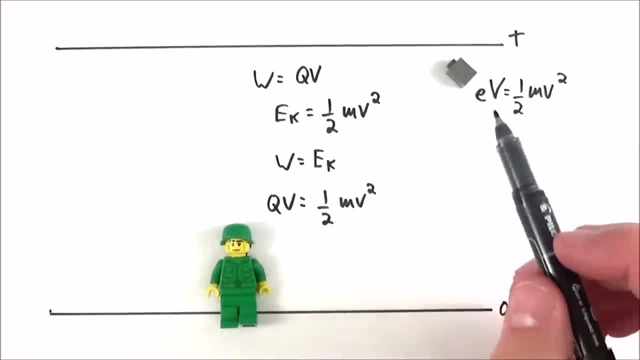 our definition of kinetic energy. So this is going to be equal to a half m v squared, And you might notice some similarities between this and our definition for the electron volt, which is in one of the other videos that I've made previously. So that's the energy that it gains, the charge. 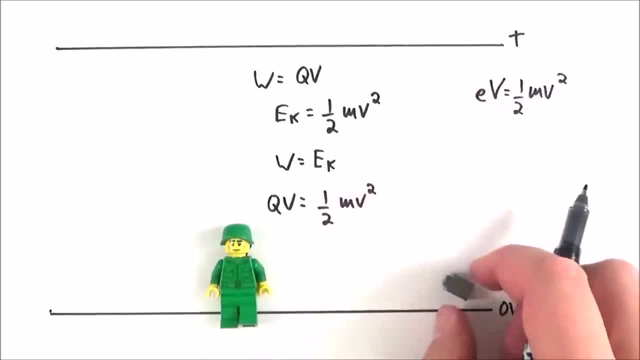 multiplied by the potential difference, And if we then release it, then this will then turn back into kinetic energy. Equally, if we apply a voltage towards this electron- perhaps it's down here- then we can accelerate the electrons by using this potential difference, And that's the 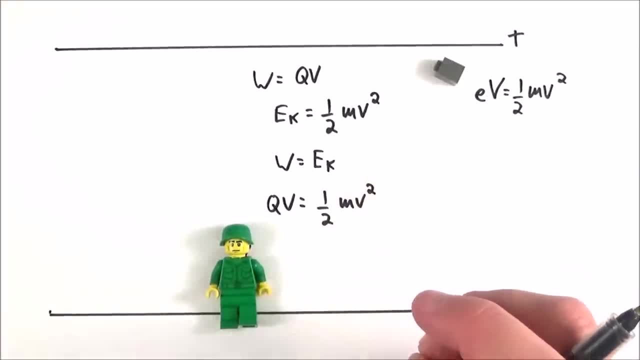 basis behind loads of things like cathode ray tubes, cathode ray oscilloscopes. We basically have these particle detectors where we accelerate particles And we can then apply a voltage to particles using a potential difference in order to give them some final energy or some final velocity. 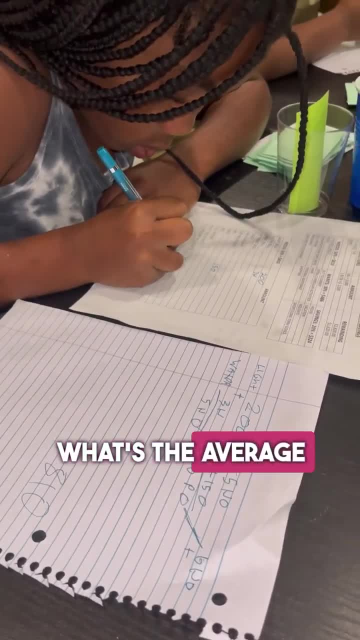 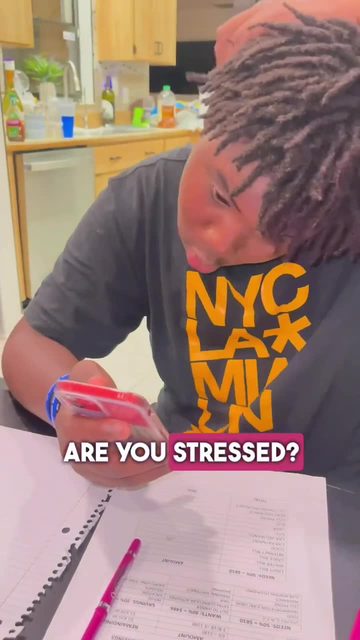 That's the average length of a car payment. You have to do your math correctly. What's the average payment for a Honda Accord 2015?? I still have no money. $339 would be your car payment. No, Are you stressed? 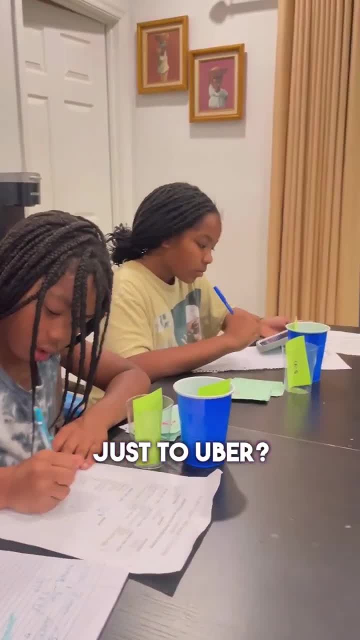 If I had a Honda Accord 2015.. Has anyone decided just to Uber? Nope, I would do what Haley did: Live in a van. I'm gonna live in a van. I'm real, Me and myself.